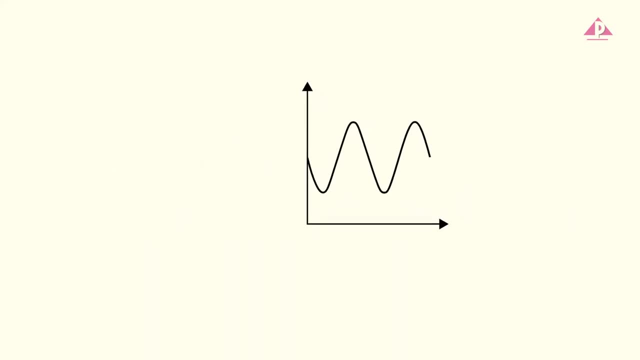 or remain constant. Point out any maximum or minimum. They usually occur when the trend changes. Let's take a look at this graph. Allen is a healthy person. This graph shows the changes in his blood glucose level after he had fasted for 12 hours and drank a glucose solution. We may divide this graph into two. 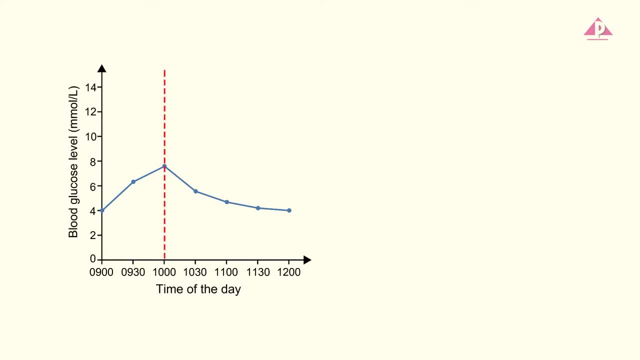 faces and mention three points. First, from 9 o'clock to 10 o'clock, Allen Alan's blood glucose level increased. Second, at 10 o'clock, his blood glucose level reached a maximum. Lastly, from 10 to 12 o'clock: 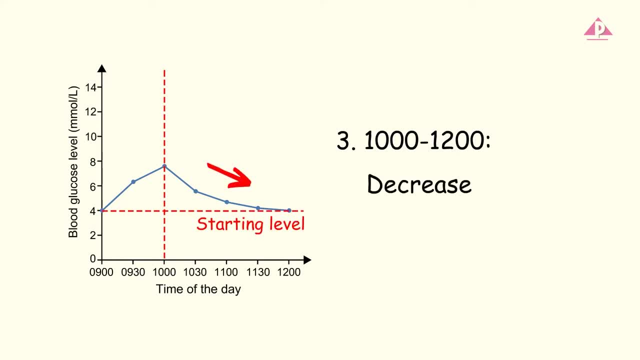 his blood glucose level decreased to roughly the starting level. Let's look at the changes in the blood glucose level of one more person. Ben is diabetic. He had fasted for 12 hours and then drank a glucose solution. The glucose solution was of equal concentration and volume as the one Alan drank. 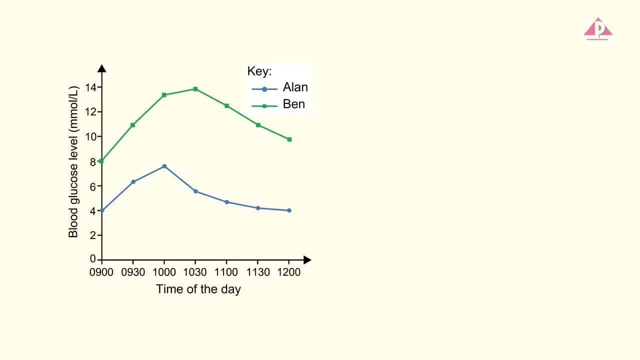 We will need to compare different sets of data shown in the same graph. What should we look for when we compare the data? First, we should compare the starting points. This graph shows that Ben's blood glucose level was already higher than Alan's at the start. 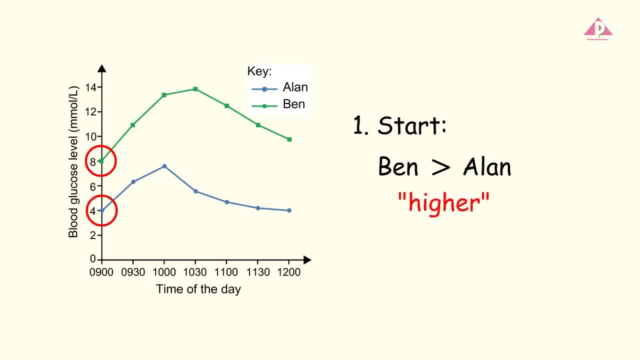 Note the use of the comparative adjective higher to clearly show the comparison. Then compare the slopes of different lines which indicate the rates at which variables increase or decrease. Ben's blood glucose level increased faster than Alan's. We should also compare the maxima. 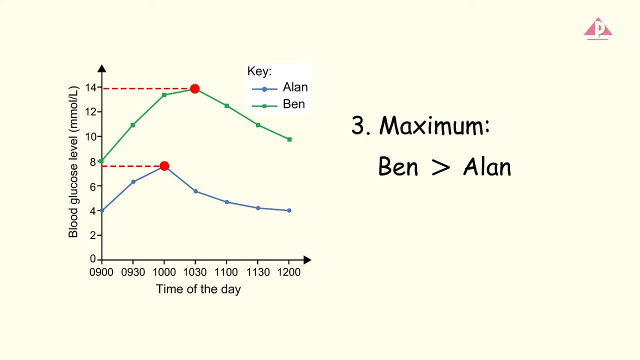 Ben's blood glucose level reached a maximum. Ben's blood glucose level reached a maximum. Ben's blood glucose level reached a higher maximum than Alan's. Then compare the time at which the maxima occur: Ben's blood glucose level reached a maximum later than Alan's. 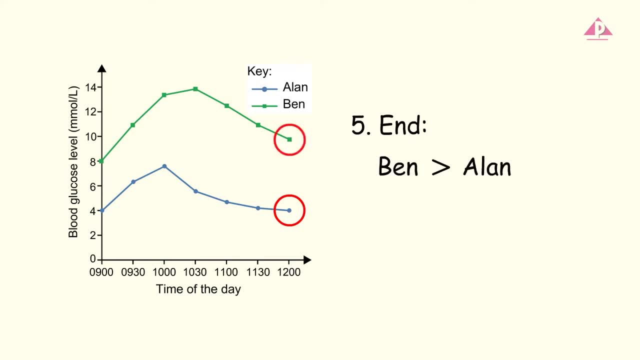 Finally, compare the ending points. Ben's blood glucose level was higher at the end and did not return to its original level as Alan's did. Some students may answer: Ben's blood glucose level returned to normal. While this statement may be true,